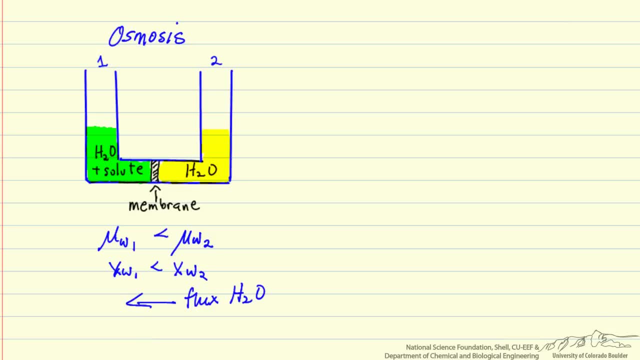 we're going to have water across this membrane from the right side to the left side to try and equalize the chemical potentials. We can also write this as the fugacity of water on the left side is less than the fugacity of water on the right side, where I've used. 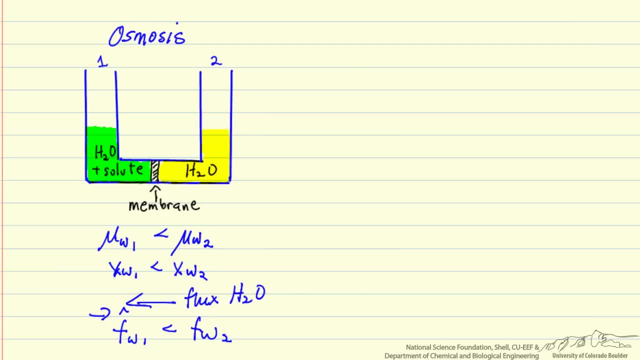 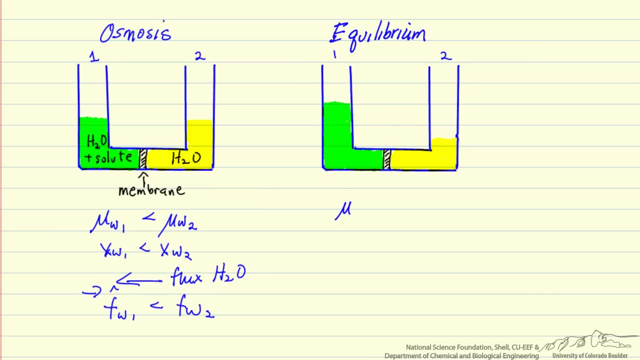 this symbol to indicate that we have a solution and on the right side is pure water. So if we let this system go to equilibrium, this drawing now represents equilibrium, which means the chemical potential of water on the left side is the same as the chemical potential of water on the right side. and 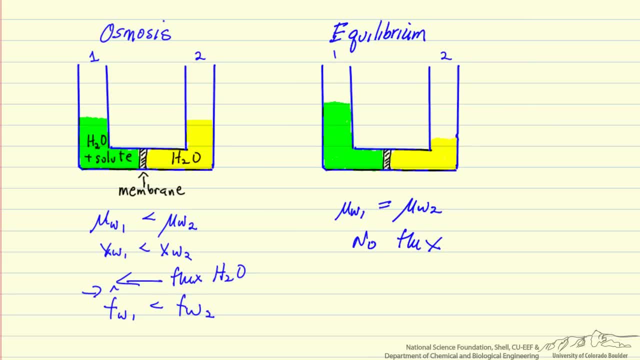 therefore, there is no flux. The way this happens is that now the pressure on the left side is greater than the pressure on the right side. As we increase the pressure, we increase the chemical potential, And then we continue to have water moving from the right to the left until we get to. 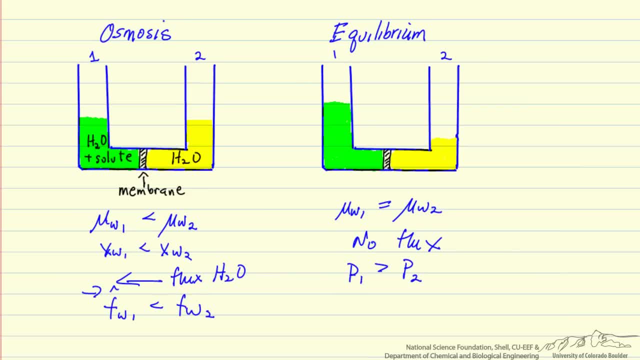 this equilibrium situation. So this delta P is the osmotic pressure. So this would be the equilibrium situation. In reverse osmosis, what we do is increase the pressure by an external means on the left side in order to permeate water to the right side. 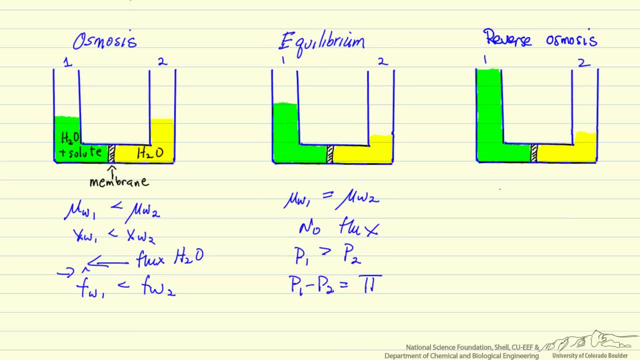 So what I've represented here in the third figure now is the idea of reverse osmosis. The idea is we've created additional pressure Here. I've shown it as hydrostatic pressure, but in reality we're going to pressurize up the liquid with a pump. And so now the chemical. 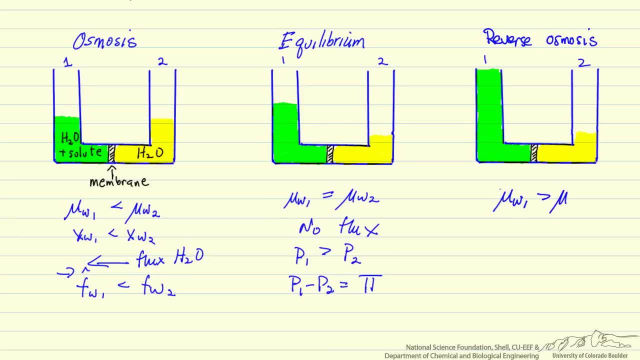 potential of water on the left side is greater than the chemical potential of water on the right side. Therefore, we're going to have flux of water on the left side And we're going to have flux of water at the station water. So the water flux is in this direction. Remember: this membrane is permeable to water. 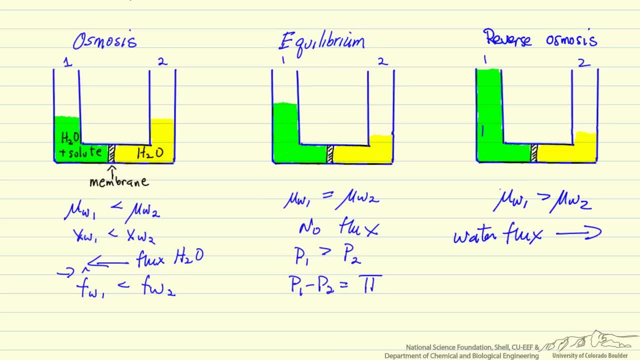 but it's almost impermeable to the salt. We have water plus salt here, and what we're going to form then is essentially pure water. on the right side, Indeed, this is the dominant process for desalinating salt water, or brackish water, meaning water with a lower concentration. 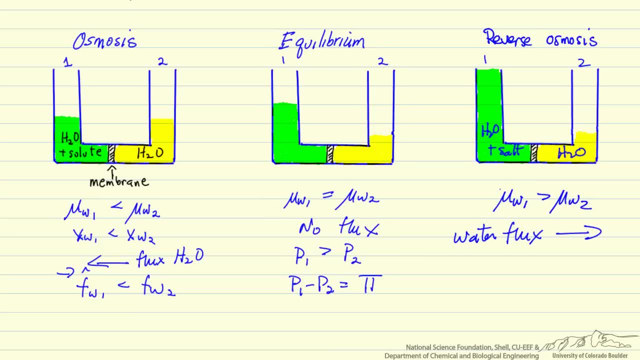 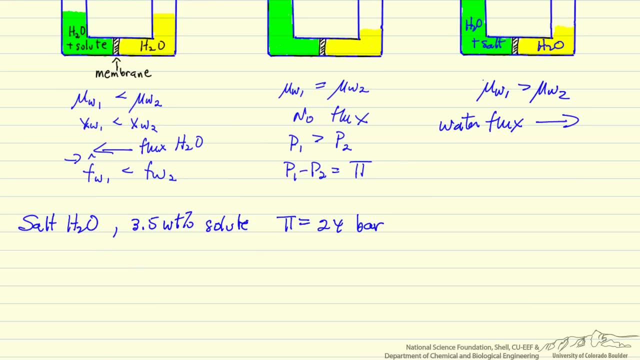 than seawater. Seawater has about three and a half weight percent of solute. It's also used to treat some food products to dewater them. So for seawater the osmotic pressure is about 24 bar. So if we're going to do reverse osmosis, that means we have to have a pressure. 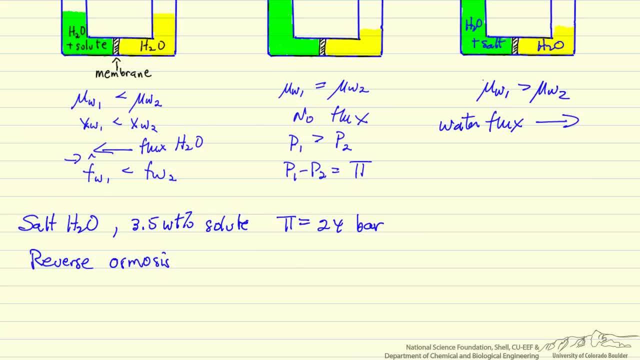 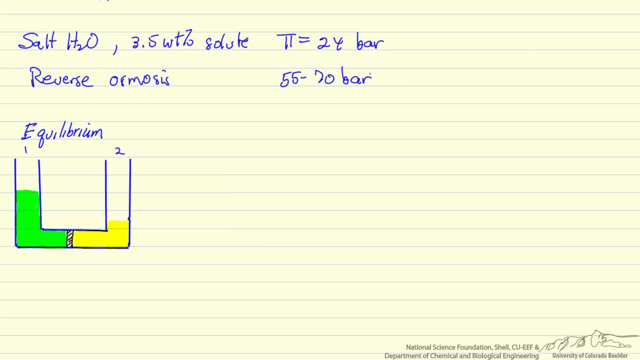 on the feed side that's higher than 24 bar, and typical values are 55 to 70 bar. So let's look at our equilibrium situation again. We have chemical potential on the left side equal to the chemical potential on the right side, and we can also 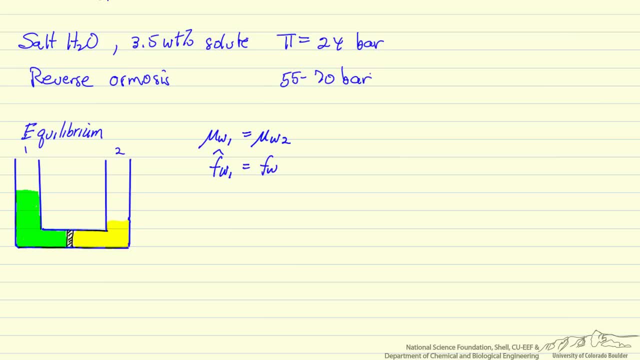 write this as: the fugacity on the left side is the fugacity on the right side And the fugacity would be the mole fraction of water and activity coefficient and then the fugacity of pure water: zero indicating pure water, and this is at pressure p1.. The right. 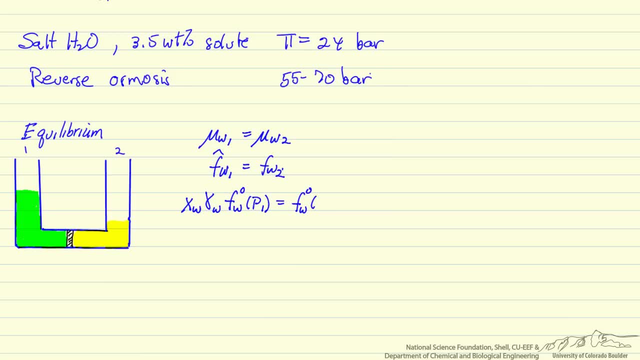 side is, we'll assume, pure water, but it's at a different pressure And then typically this is going to be close to one, because this is close to one. If this were 0.98, for example, it's a pretty good approximation that the activity coefficient is close to one. So we 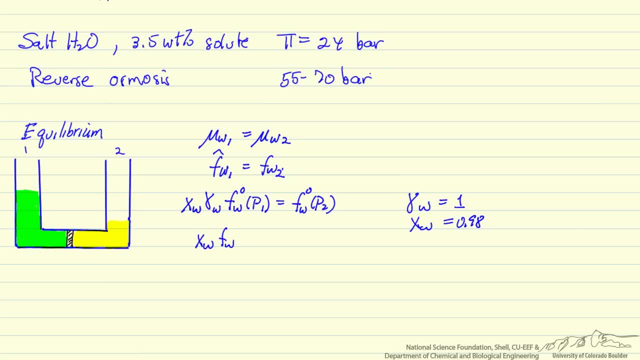 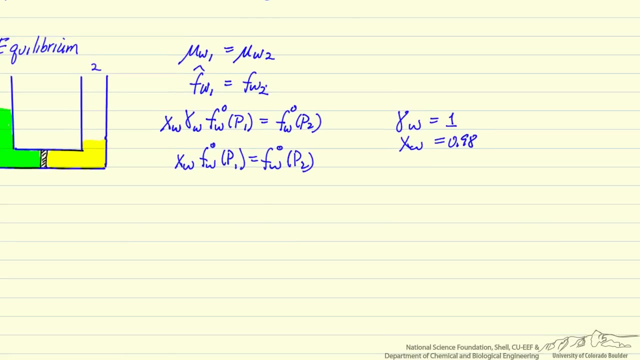 have the mole fraction of water times the fugacity of pure water at this pressure, equal fugacity of the different pressures. And so what we're going to use to relate the fugacities at the different pressures is the pointing correction. So this is the pointing correction. 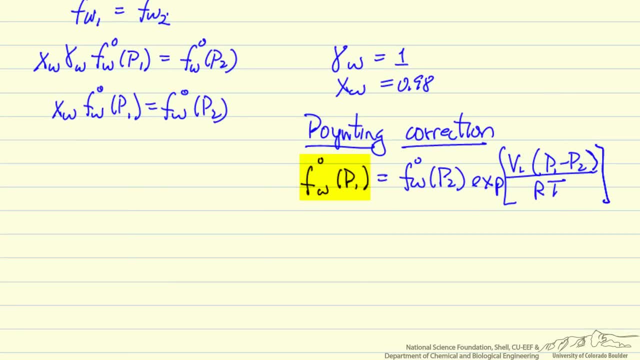 It says the fugacity at pressure p1 for pure water is equal to the fugacity of pressure p2 times an exponential Pressure difference. This term is the volume per mole of the liquid Gas, constant and absolute temperature. We've been talking here about equilibrium, which means p1 minus p2 is our 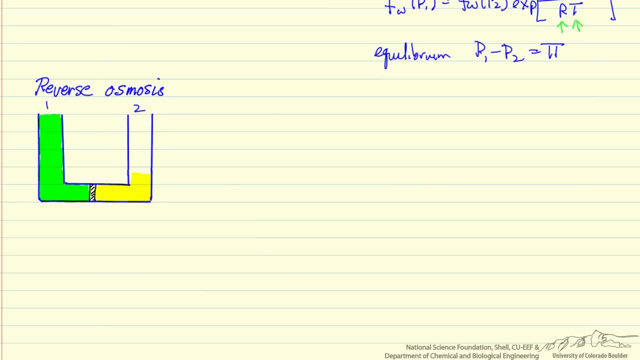 osmotic pressure. So now let's look at reverse osmosis. So we're going to have water permeating through the membrane in this direction: The flux of the water. So this is flux Moles per area, per time, The flux of the water. 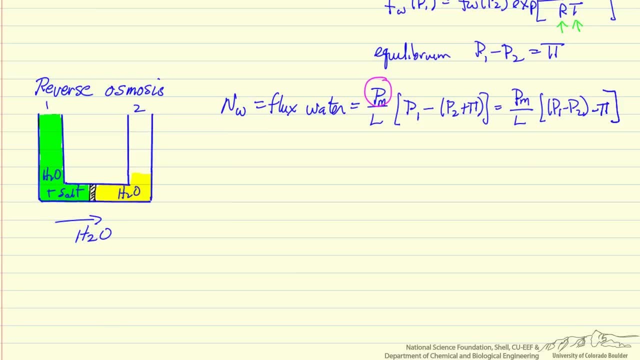 So the flux, it turns out, is proportional to permeability. This is a property of the membrane Thickness. Thicker membrane has a lower flux. And then the pressure on the feed side minus this quantity. The pressure on the feed side plus the osmotic pressure, Because, remember, if this pressure 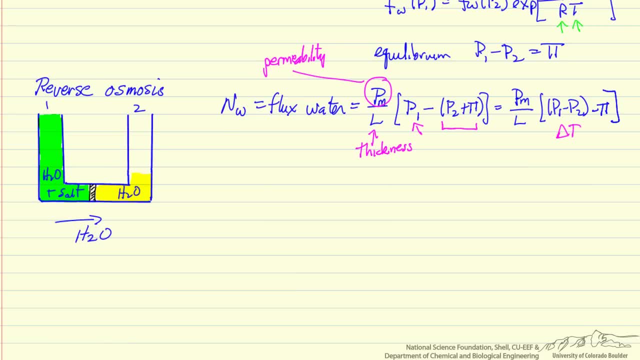 difference, so this we'll call this. pressure difference across the membrane was equal to the osmotic pressure, it would be no flux. So we have to have a pressure difference greater than the osmotic pressure to have reverse osmosis. So here's the equation for the water flux: Higher pressure on the feed side, higher pressure. 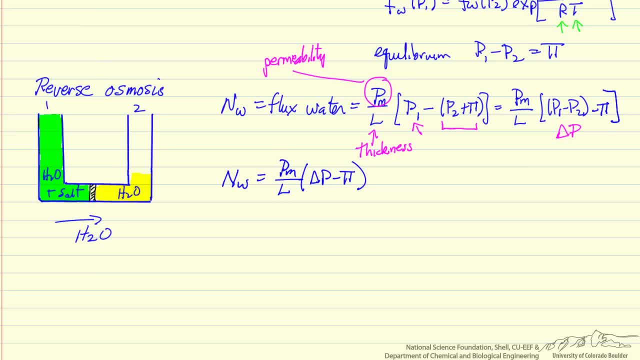 on the feed side, We could have a small amount of salt, Not a perfect membrane, So we could also look at the flux of the salt, Which would be related to the diffusivity of the salt in the membrane, Again divided by the membrane thickness. 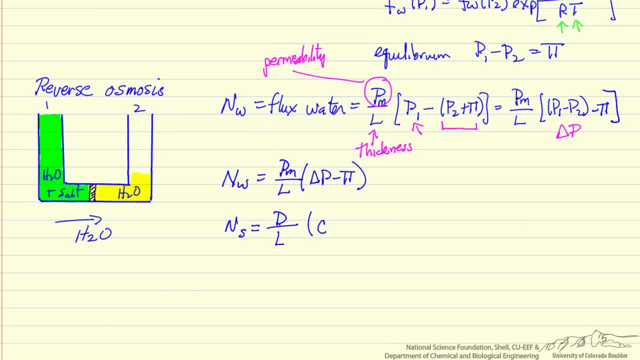 Now we would have the concentration of the salt. This would be on in the membrane right at the edge. So the membrane, your side 1 and side 2, that would be the concentration right here. call that prime and then the concentration right here. 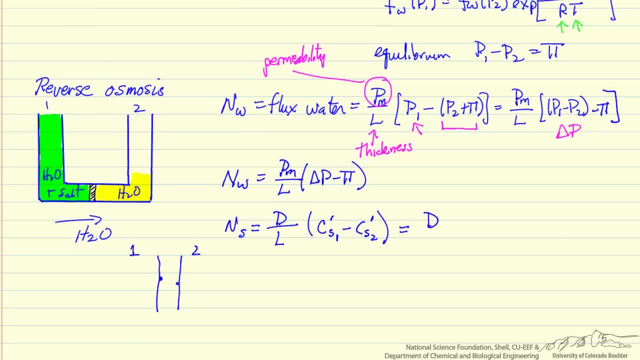 And what we can do is relate this to a partition coefficient for the solute and then write the concentrations in solution. So these now are the concentrations. this is liquid salt plus water, side 1, this is almost pure water, but a very low concentration of salt.